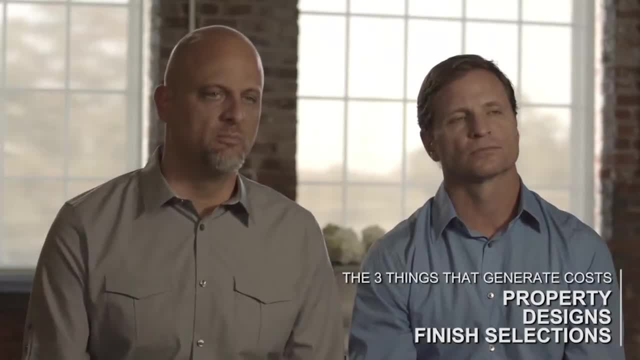 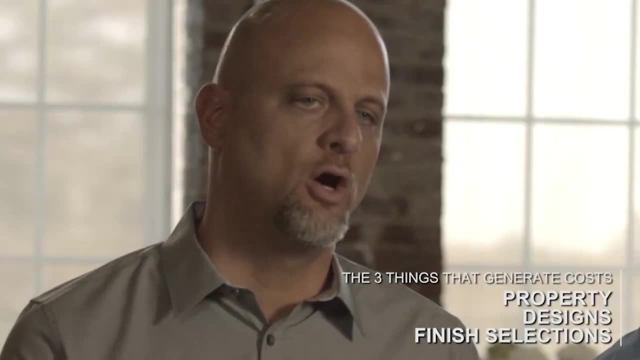 is the homeowner's finished selections, And these three things must be controlled, because they control the outcome of costs across the entire process, And the problem is that homeowners don't know how to control these, So therefore they have to let other people control it for them. 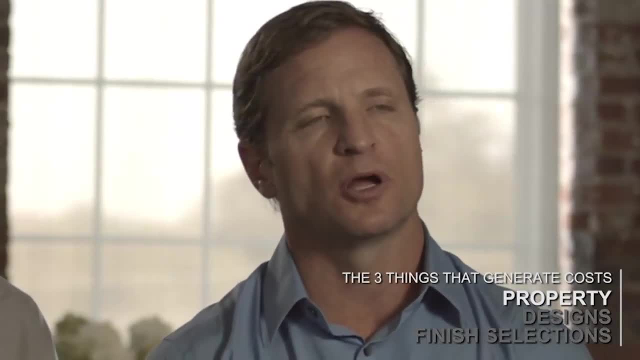 And the first factor is that lot Most homeowners don't understand how much money can be lost if the wrong design is set up with the wrong lot. There are thousands, tens to hundreds of thousands of dollars sometimes that can be lost by pairing up the wrong plan. 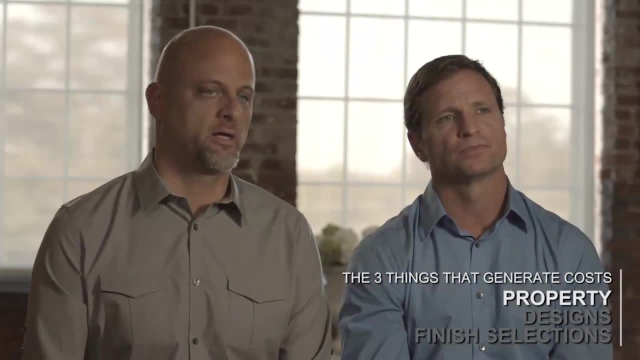 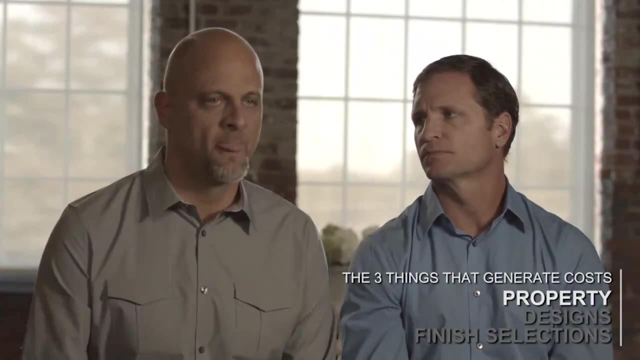 with the wrong property. That's right, Lee, And so most homeowners don't know how to control the design. They have to let someone else control it for them, And I had a client, for example, that had a very steep mountainside lot. 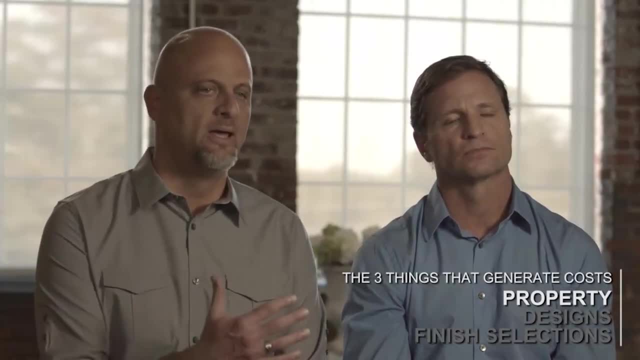 And she wanted this plan that I had designed as a wonderful plan. but I had warned her this is gonna cost a lot more than you think it will, because of the foundation wasn't right for the lot. Well, sure enough, the builder priced out the construction documents. and discovered they had a $200,000 increase in the foundation cost of the home, And so we had to redesign the whole plan over again. but it was all because the homeowner simply didn't understand the cost impact of a plan- a good plan on the wrong lot. 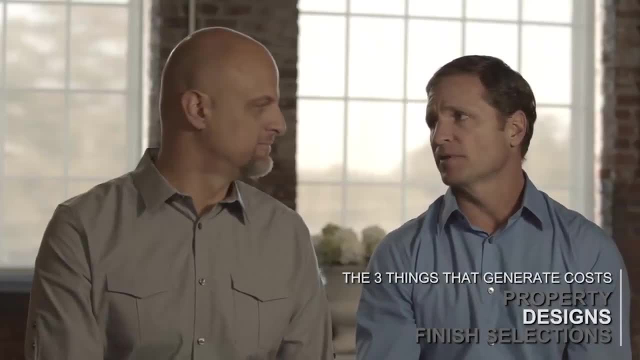 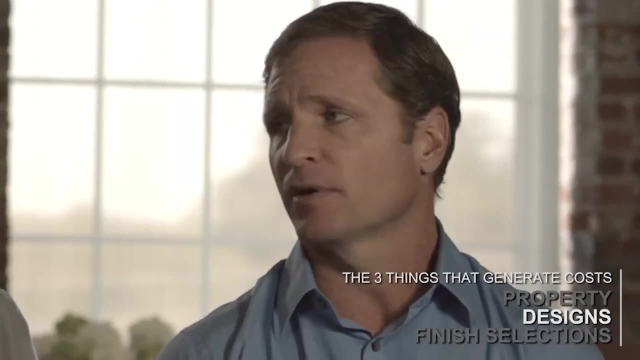 And then the second cost factor. we've talked about the property. the second cost factor is just the design itself. Most homeowners don't realize that square footage can have different costs depending on where it is, That the first floor of a house is so much more expensive. 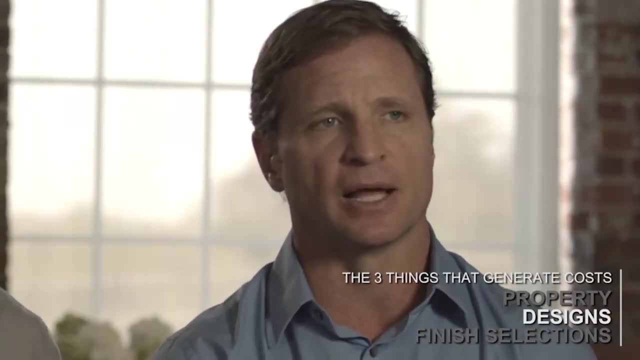 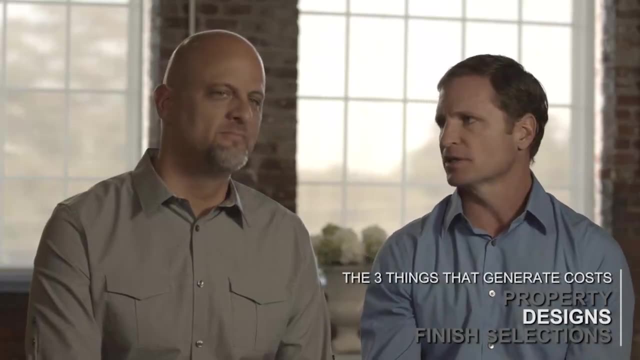 than going up or going down. So most times clients want this sprawling house and that's fine if that's what they want. but we want them to understand what those cost implications are, And if not, sometimes costs can just get way out of hand. 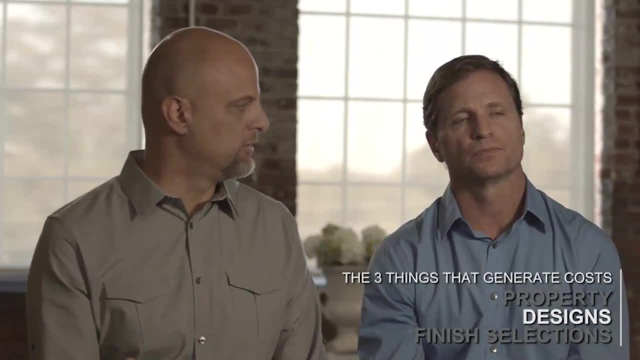 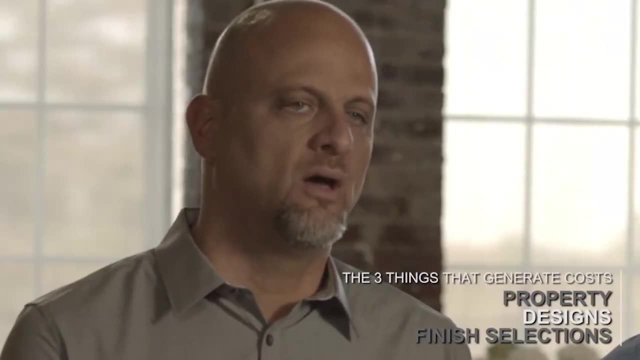 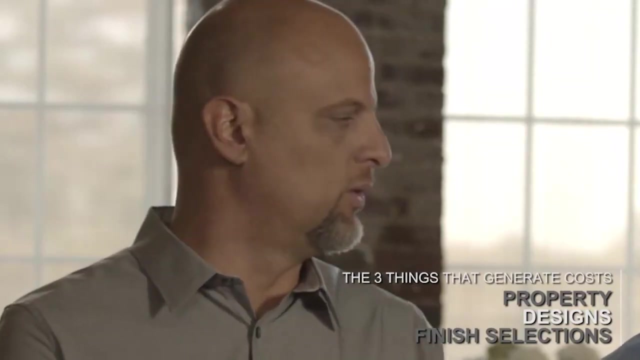 That's right, and so homeowners need to know how to balance this square footage versus complexity of plan factor to homes, And so so often homeowners want a big, sprawling main level And, like you said, Lee, that's fine, but the square footage cost is gonna go up. 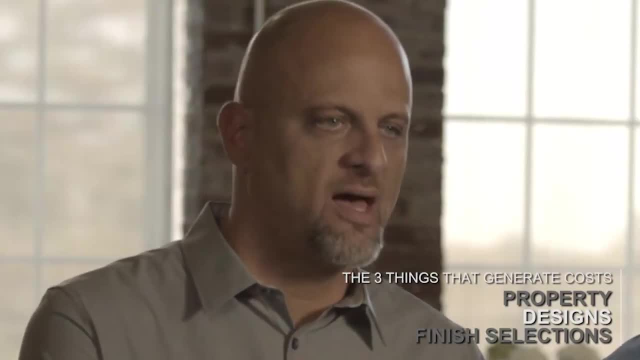 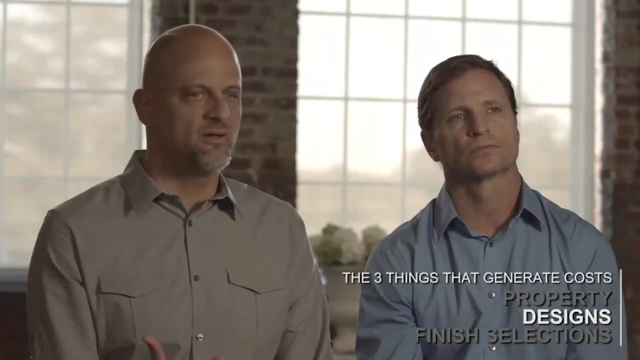 And so homeowners just need to be aware of how to balance the size of a home with the costs that they wanna spend on building this thing eventually, And so sometimes it requires simplifying a design or reducing the complexity of it. It's just that homeowners need to understand. 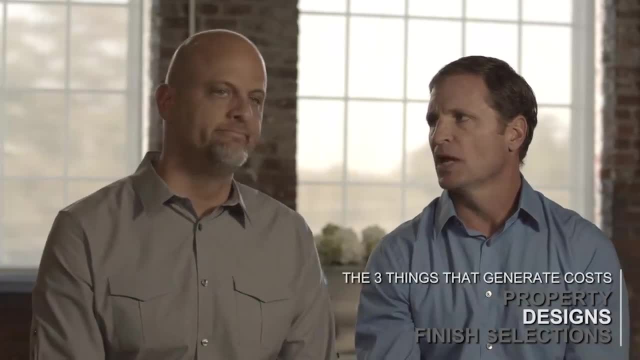 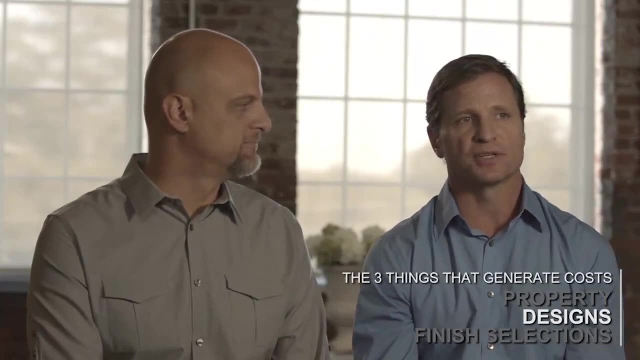 the balancing act of their design priorities versus their budget And, like you said, at the end of the day we're just wanna have an informed client. Somebody can make a decision that they understand. hey, if I'm gonna have my house more sprawling, 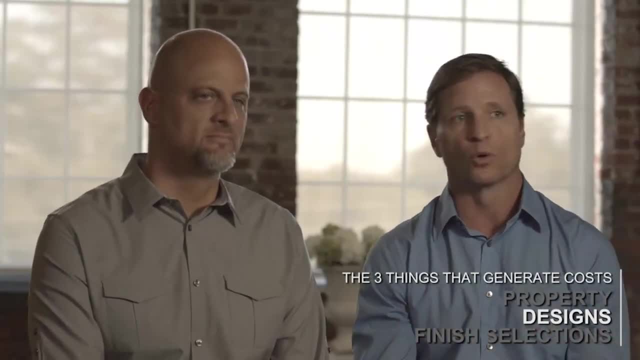 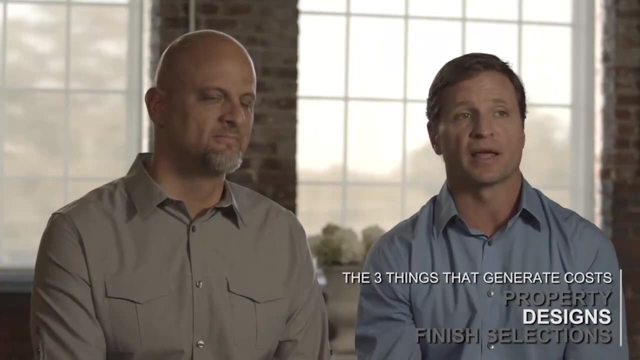 or more complex design, more curves, more corners, more roof designs, whatever it might be. that's gonna drive cost, And if that's where they wanna spend their money, that's of course fine. We just want them to understand that going into it. That's right. Building always controls cost. The builder doesn't control cost, It's always the design, And so only the homeowner can control that process with their architect. Now again, we're not saying homeowners can't have beautiful custom homes. 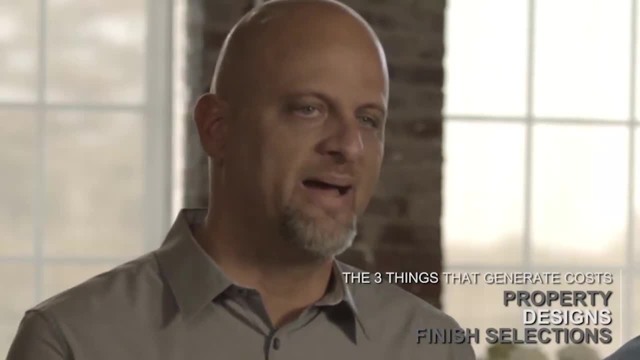 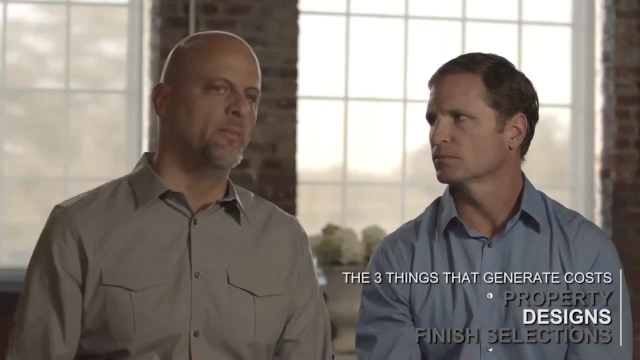 We do it all the time, but we help our homeowners balance beauty with efficiency, And that's where the homeowner needs to direct the architect, because architects like to be creative, which makes the cost go up. Builders like to be efficient, which can take away a little bit of the beauty. 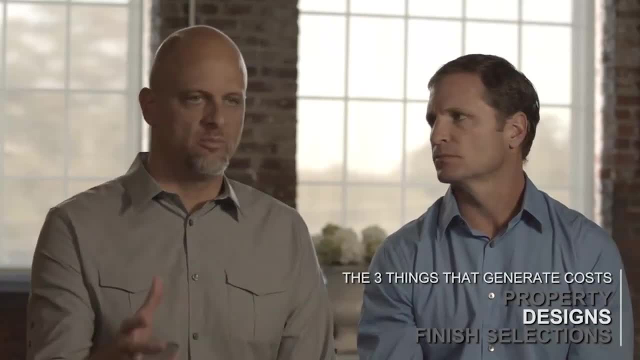 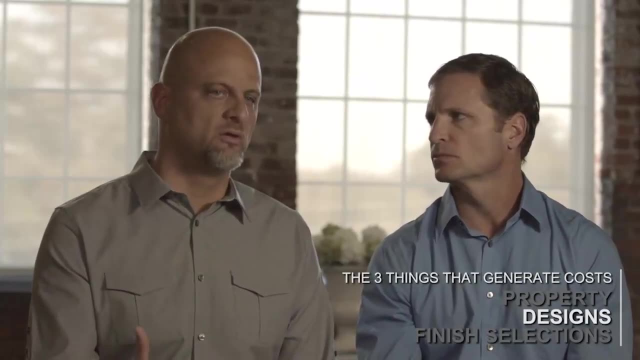 Only the homeowner can control that balance Between the architect, the builder, the designs. And so homeowners need to learn these processes, need to learn these secrets to control the outcome of their dream home investment. And then that just leads us to really the third cost factor. 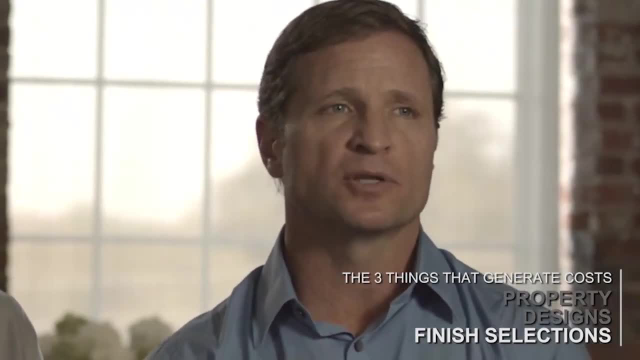 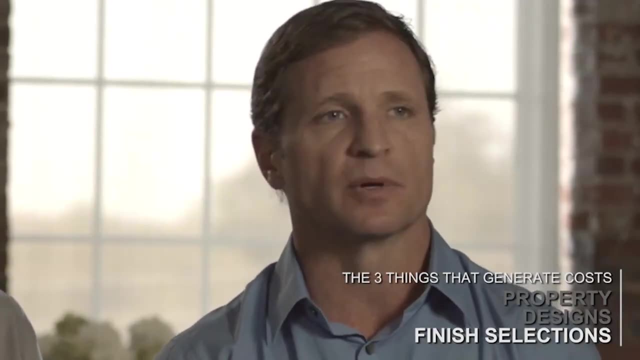 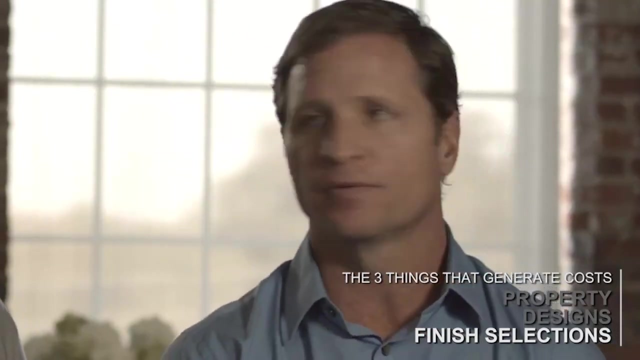 which is the selections, And again, an area that most homeowners really do not understand- what a huge impact that their selections have on the price per square foot. And, at the end of the day again, we want the client to get the appliances that they want or the roof that they want. 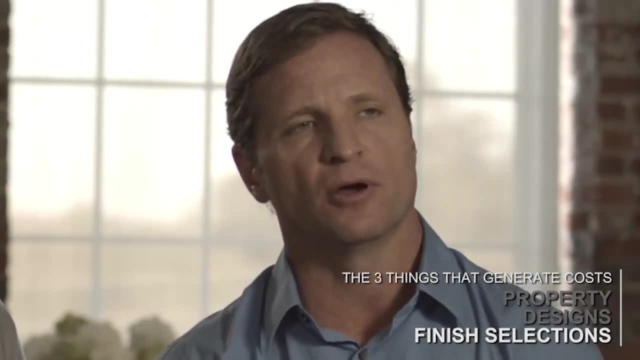 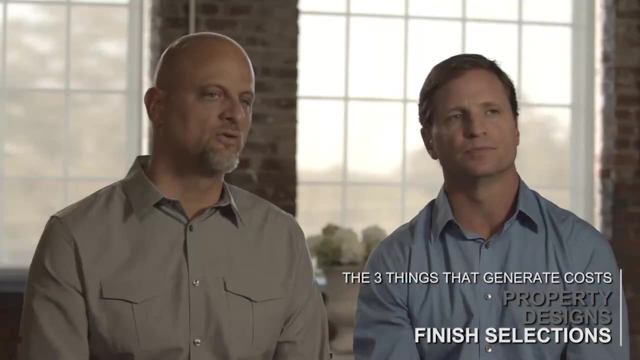 or whatever it might be, But we just want to make sure that the homeowner understands that making these selections will ultimately determine where that cost per square foot will be. That's right, Because only the homeowner can control costs for their home And these finished selections are entirely. 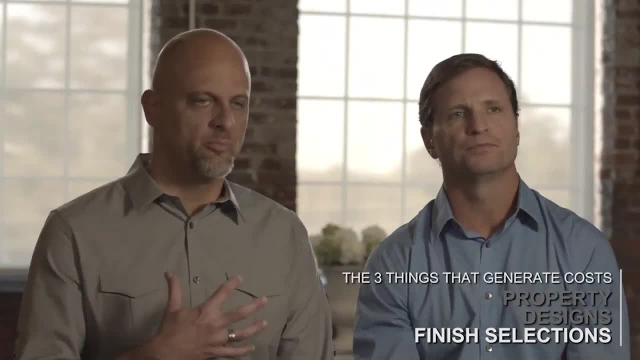 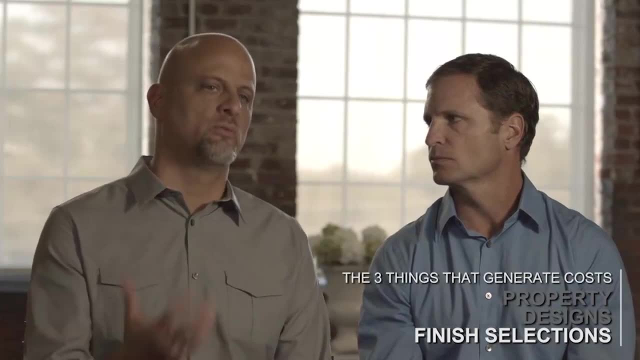 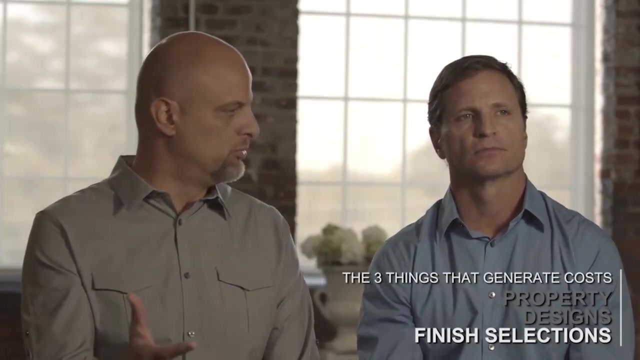 within the homeowner's control because it's their emotional and personal selection. Obviously, the higher end finishes cost more, So there's a couple of solutions that we always offer If you have a smaller home. that's a simpler design, still beautiful, that actually makes room. 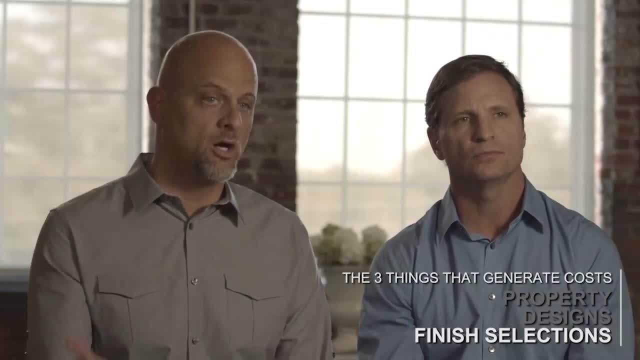 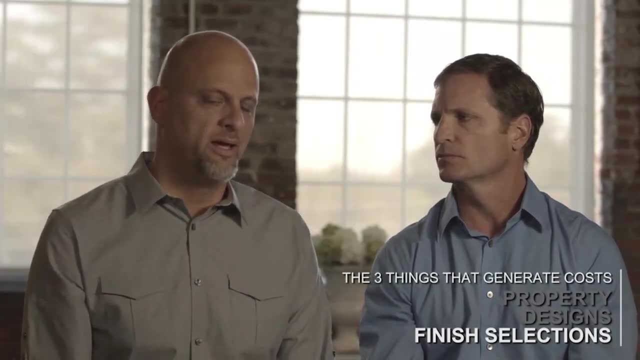 for more expensive, more high-end finishes, But a large, complex design reduces the amount of nice finishes or has to reduce the quality of the home, And so the homeowner needs to learn how to direct the architect and the builder to achieve the ultimate outcome they really want. 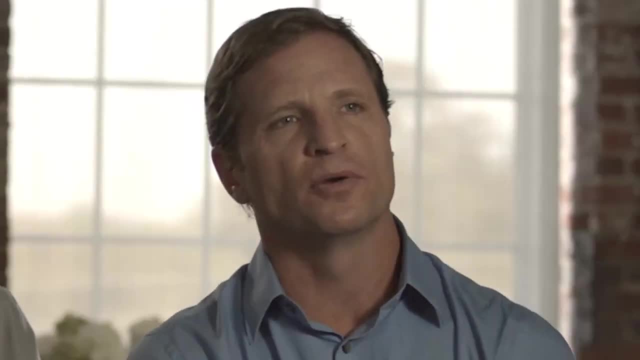 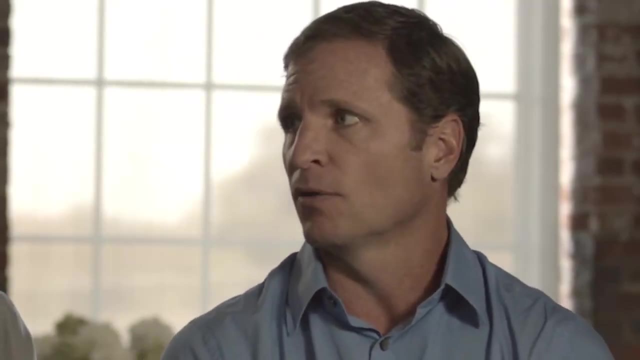 And the problem is most homeowners don't know how to do that And most homeowners let the architect, the builder or the interior designer control the process, And the challenge is they don't realize that usually that leads to an over budgeted home. 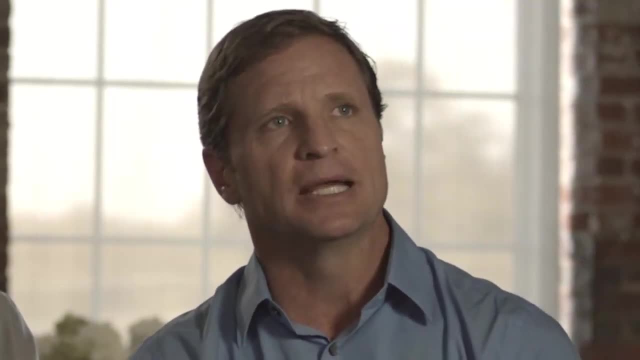 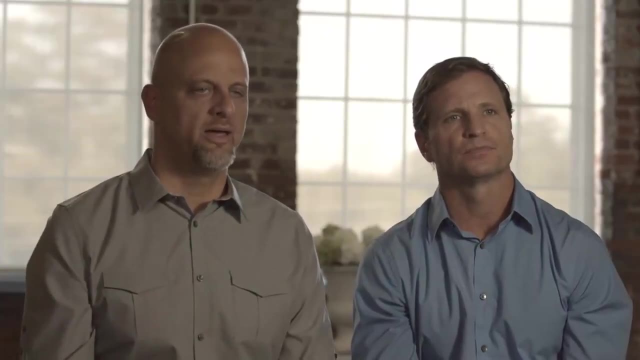 And this does not have to happen. I mean, the homeowners can direct the process well enough to where design can meet a budget. That's right, Because design does control every outcome here, And so if the designs are over budget, everything else is gonna follow. 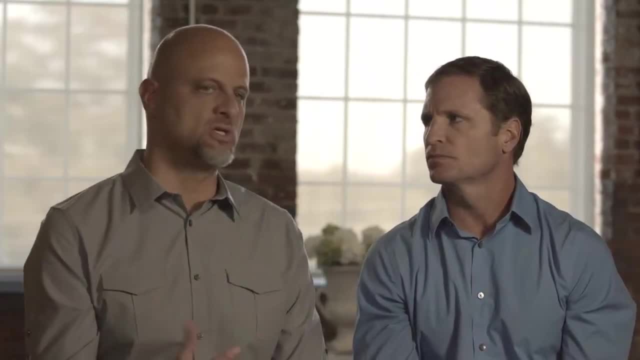 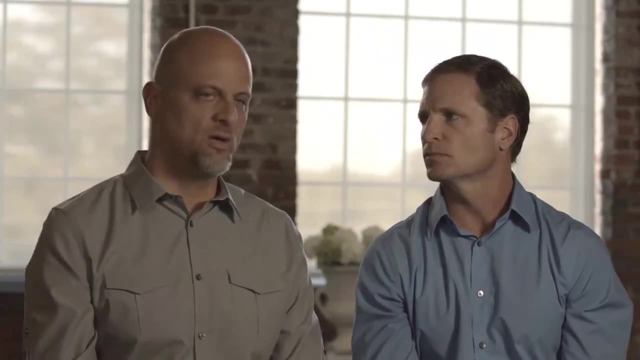 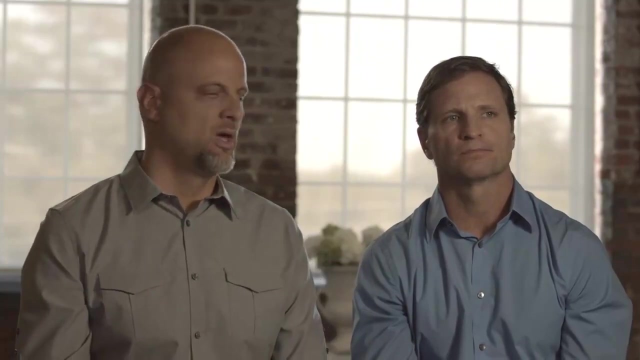 And so we've created what we call an on-budget strategy. that must be followed. It gives homeowners the information and the plan and the process to achieve the home that they want and the budget that they expect, But it must start before designs begin, before they sign any agreements. 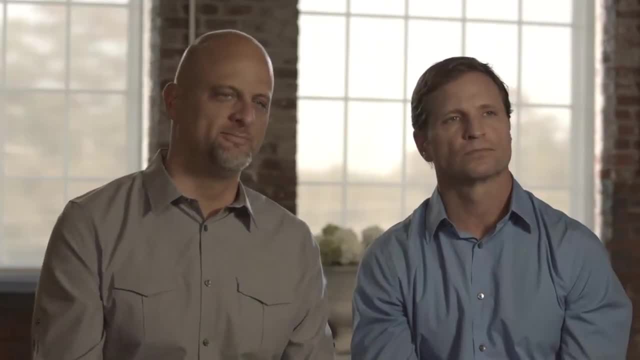 And that way the homeowner will be in control right from the start. 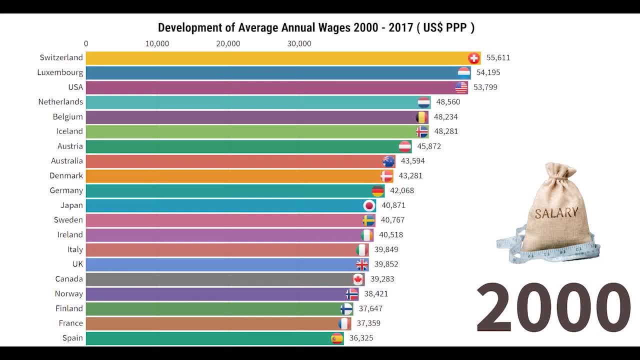 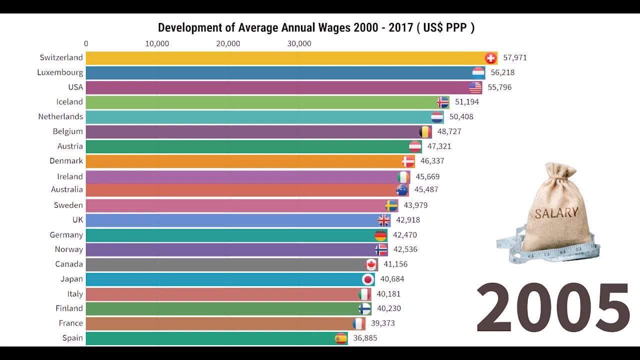 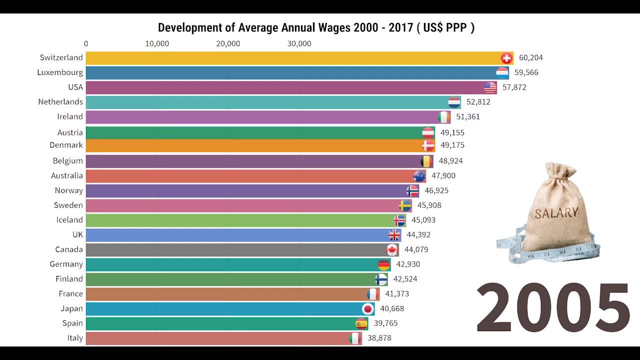 The average wage is a measure of total income after taxes, divided by total number of employees employed. In this video, the average wage is adjusted for living expenses. purchasing power parity- PPP. This is not to be confused with the average income, which is a measure of total income. 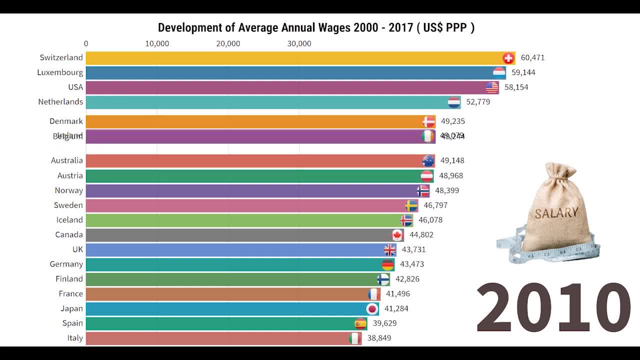 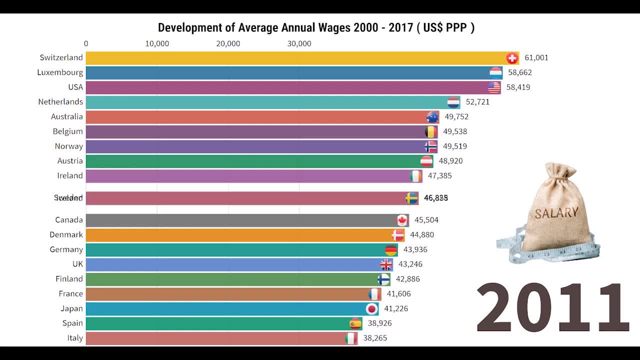 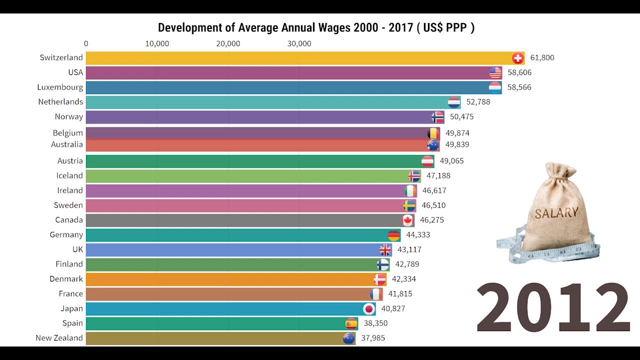 including wage, investment benefit and other capital gains. divided by total number of people in the population, including non-working residents, The wage distribution is right skewed. the majority of people earn less than the average wage. For an alternative measure, the median household income uses median instead of average. The OECD Organization for Economic 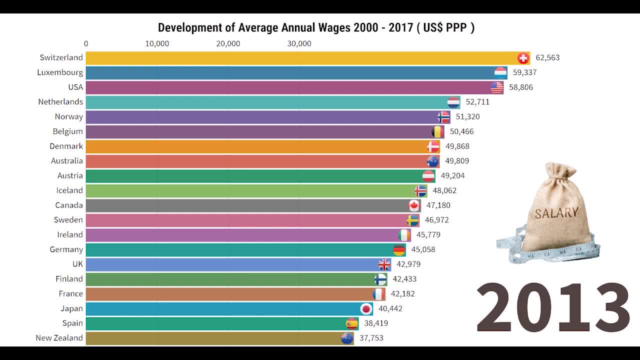 Cooperation and Development. DATASET contains data on average annual wages for full-time and full-year equivalent employees in the total economy. Average annual wages per full time and full-year equivalent employees in the total economy. Average annual wages per full-time equivalent dependent employee are obtained by dividing the national account space: total wage. 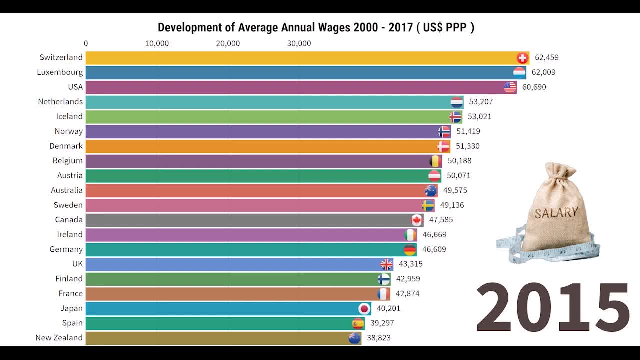 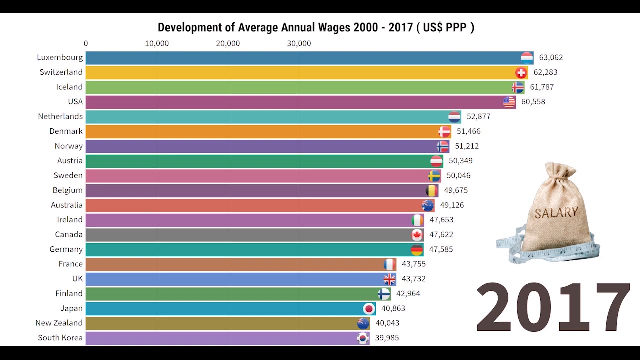 bill by the average number of employees in the total economy, which is then multiplied by the ratio of average usual weekly hours per full-time employee to average usually weekly hours for all employees. One of the most significantcićr score was in the US.